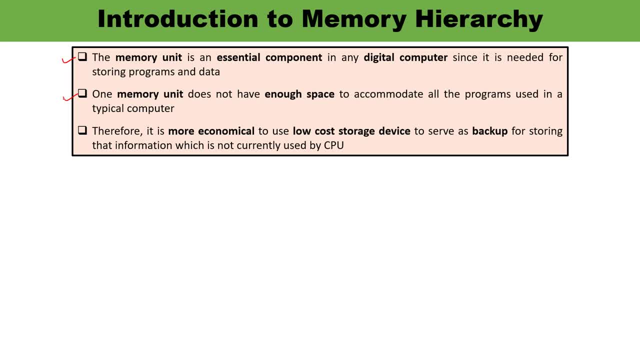 space so that they can accommodate all the programs in a typical computers. or you can say it is also more economical to use low cost storage device, right that can serve as a backup. also means you use to use a term- backup means to store your required information which is not like available currently. 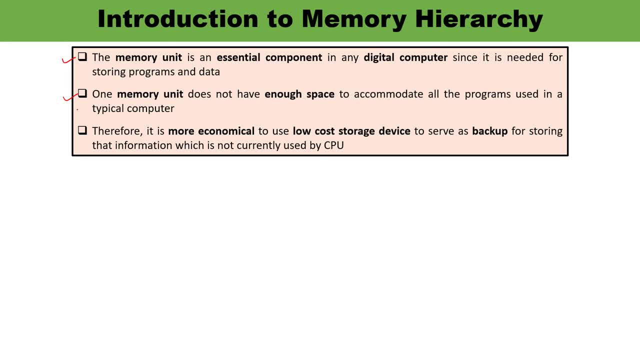 used by the cpu and whenever you require you can access that particular device. it means low cost storage device can serve as a backup. that is also very important here. you can see in this particular diagram you can observe the components of a typical memory hierarchy. so there are various components, as you can see: auxiliary memory, io processors, cpu. 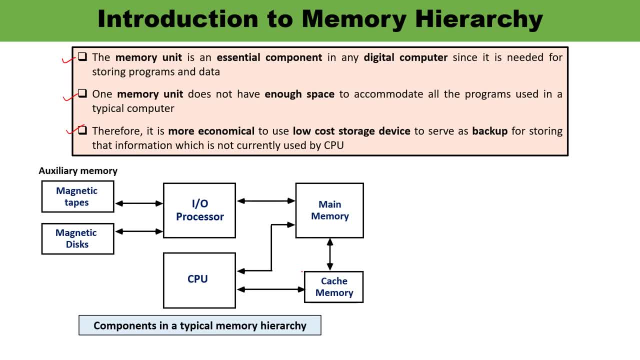 main memory and cache memory. so let me give you a brief about it. see the memory unit which communicates directly with the cpu- that is known as a main memory, and the device which provides backup storage right- that is known as a auxiliary memory. backup storage means magnetic tapes. 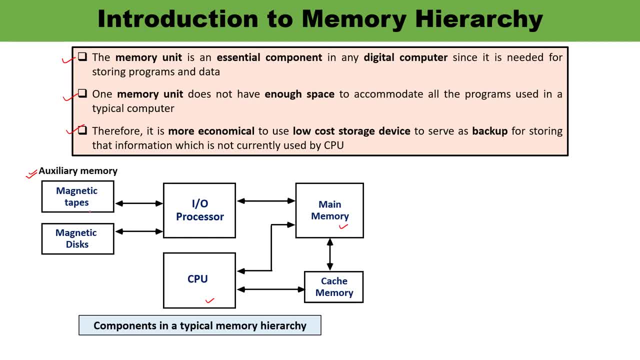 magnetic disk can be used as a backup space, so auxiliary memory. they are used for storing some programs or sometimes large data files or other backups. so only the programs and data which is currently needed by the processor. that retains in the main memory means whatever is being required by the. 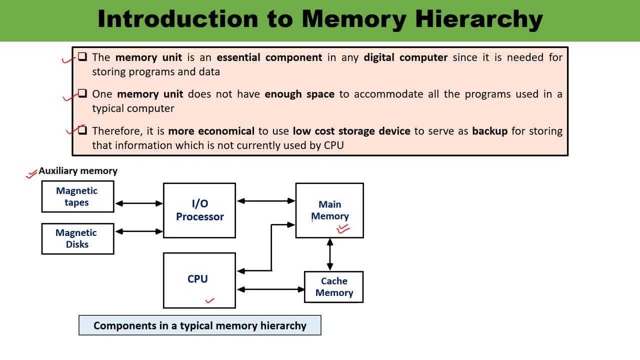 processor that will be available in the main memory and all other information can be stored in the auxiliary memory and that can be transferred whenever required to the main memory. so, as i have told you that this shows the some basic components which are the important components over here, so you can see in this particular diagram the main. 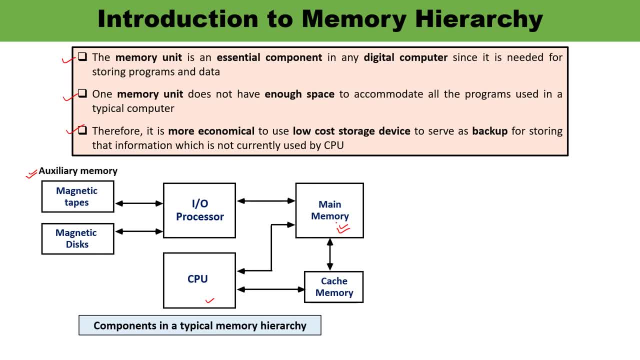 memory. it occupies a central position over here. central position means in terms of it can. it is capable to communicate directly with the cpu and with the auxiliary memory via io processor. so main memory can communicate with cpu as well as the auxiliary memory. also. it means when programs not 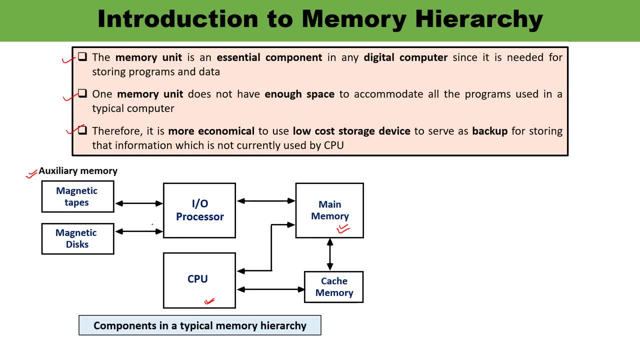 residing in main memory right means when the programs are not available in the main memory, they are brought from the auxiliary memory via io right. and here you can see one more term, which is the cache memory. see, this is a special, very high speed memory, cache memory- and sometimes it is used to increase the speed of the 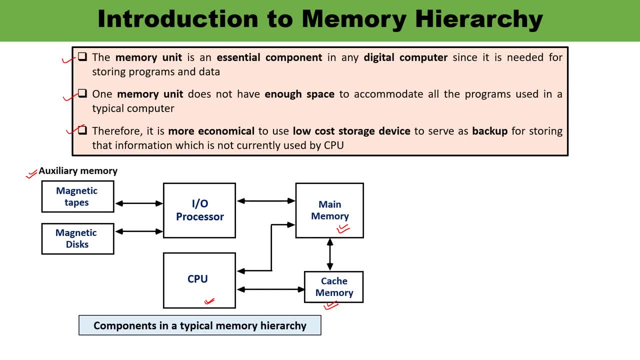 processing, you must have heard. and the cache memory is employed in computer system basically to compensate for memory of the processor whenever there are the speed difference in between the various other units. like the speed will be different for the main memory, speed will be different for the CPU and all it means there. 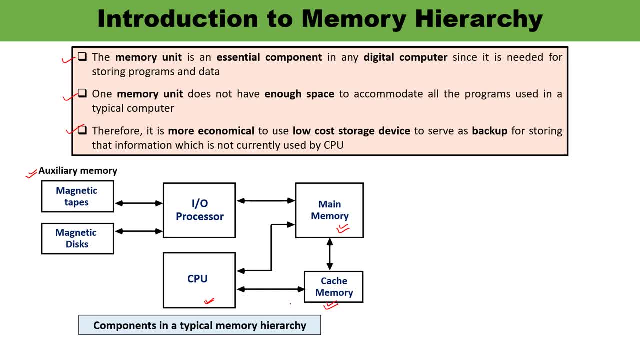 is a requirement of a technique which is used to compensate the mismatch of operating speed right, and that mismatch can be handled when CPU, when cache is used. so cache, there is a that this is a kind of small cache and that is kept in between the CPU and the main. 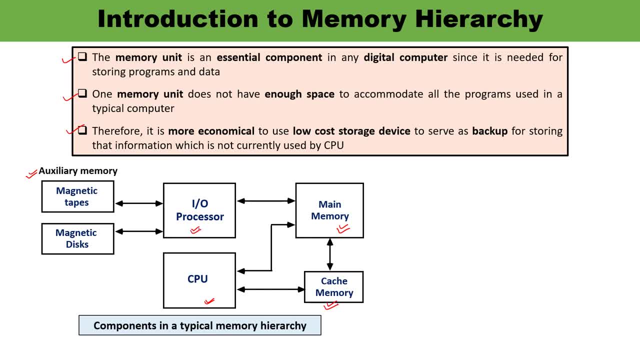 memory and, as you can see here, IO processor, input output processor. it manages data transfer between auxiliary memory and main memory and the cache organization is concerned with transfer of information between main memory and the CPU. I hope now this particular point must be clear and you must be aware that this auxiliary memory, auxiliary memory- it is having a large storage capacity. 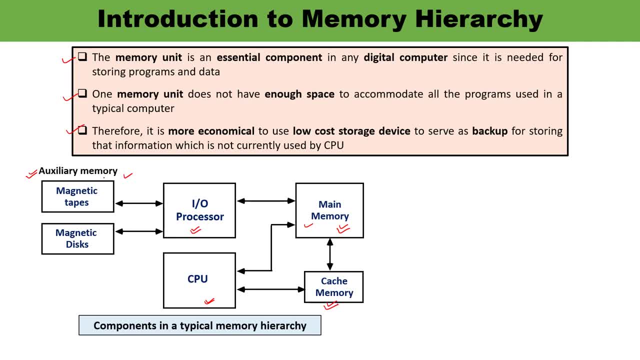 right and it is relatively inexpensive also. but here it has low excess speed in comparison to the main memory. so the excess speed of auxiliary memory is less and the cache memory. this is very small, so it is relatively expensive also but it has very high, high excess speed right. so overall, 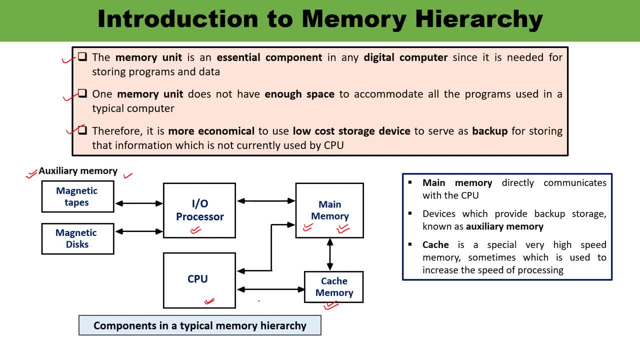 goal of using a memory hierarchy is to obtain highest possible average excess and, at the same time, minimize the total cost of the entire memory system. that is why it is being required- and let me tell you one more point- that auxiliary and cache memory. both are having the different purposes. like the cache, 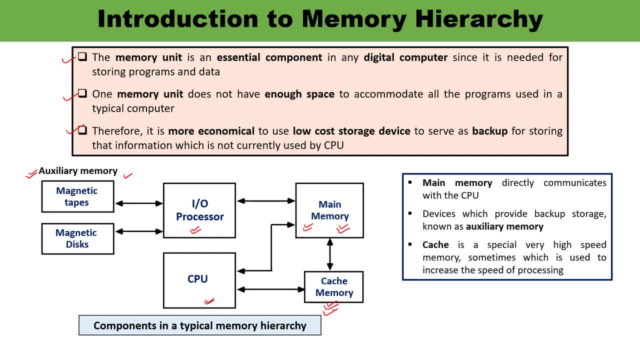 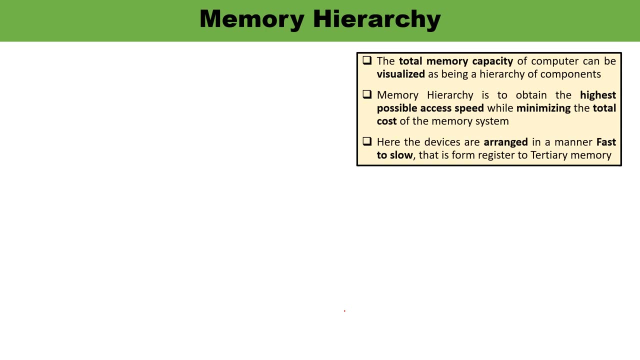 memory, it holds those parts of the program and data which are most heavily used, while auxiliary memory it holds those parts that are not presently used by the CPU means it is not presently used by the CPU, but this is heavily used. Now let us, uh, draw a memory hierarchy system. so when you can draw the memory hierarchy, it is. 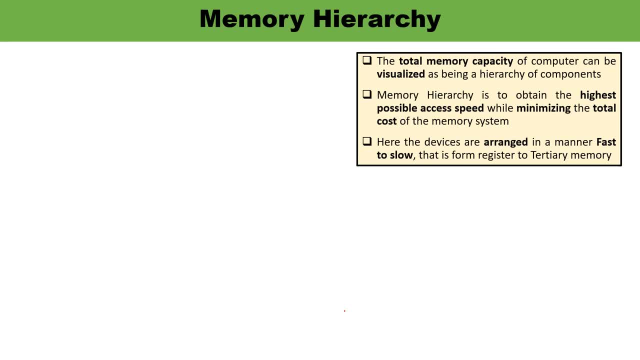 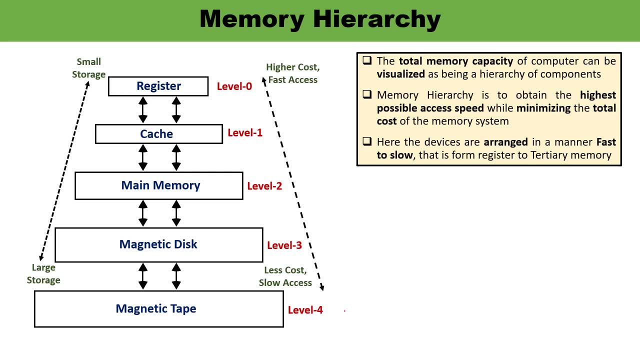 actually being divided into five levels depending upon the speed and use. so here the processor can move from one level to the another level based on its speed requirement. and these five hierarchies in the mammaries you can observe: register, cache, main mammary, magnetic disk and magnetic tapes. So the total mammary capacity you can visualize. 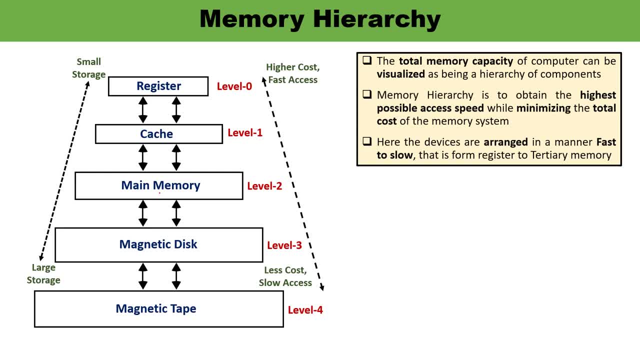 as a mammary hierarchy. right and as you can observe over here there are important two terms: which is volatile and non-volatile. So the first three hierarchies which we are talking about: register, cache and main mammary. These are the volatile mammaries, means they can lose the data. 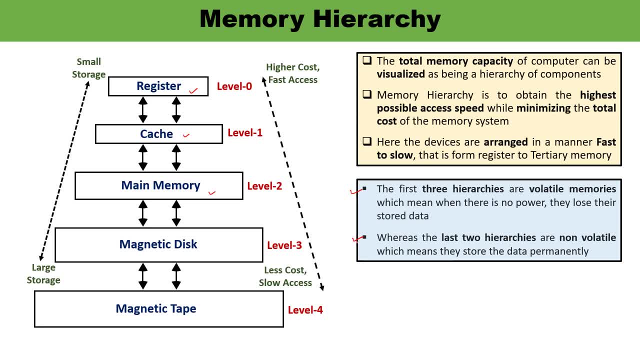 whenever there is a power off, while the other two mammaries last two: magnetic disk and magnetic tape. they are non-volatile, means they can permanently store the data. Here, these three level 0, 1, 2 means register, cache and main mammary. It is also known as a internal mammary because this is 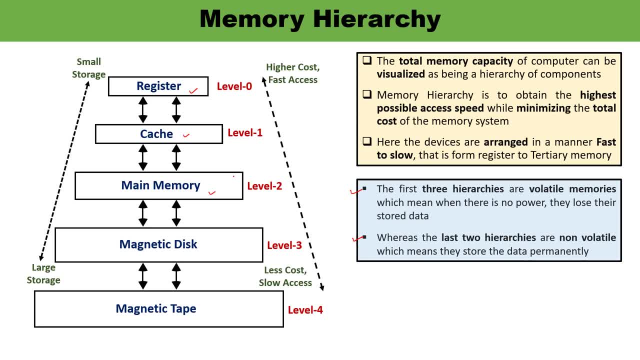 accessible by the process of storing the data. So this is the process of storing the data. So the two mammaries is one and the One is the process of storing the data. This is called the acceptor. you canerella, As you can understand. All the three confian密ど not enroll in the 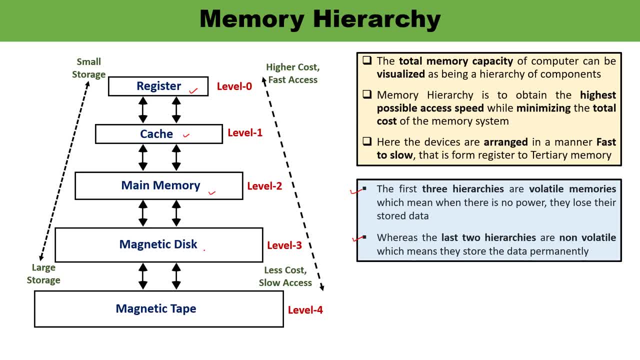 process of storing the data, you have to transfer this data to the processor directly, and this mammary contains these three parts, while there is one more term which is about the secondary mammary. Secondary mammary is also known as the external mammary, means primary mammary or internal. 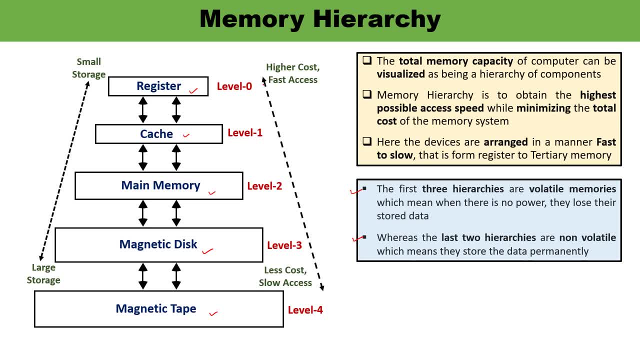 me give you one in detail the explanation. as you can see, on the higher side here, the cost per bit. we are talking about higher cost, fast excess cost is higher because per bit why when you are moving downward it gives you less cost and slow excess at the same time. storage. 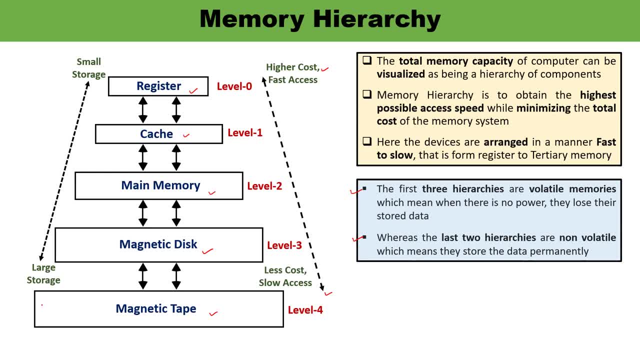 capacity of registers is small in comparison to the storage capacity of the magnetic tape that is being like shown over here. so let me give you in detail. when we are talking about level zero, level zero means register. so here, at some of the places you must see the term CPU. so actually, 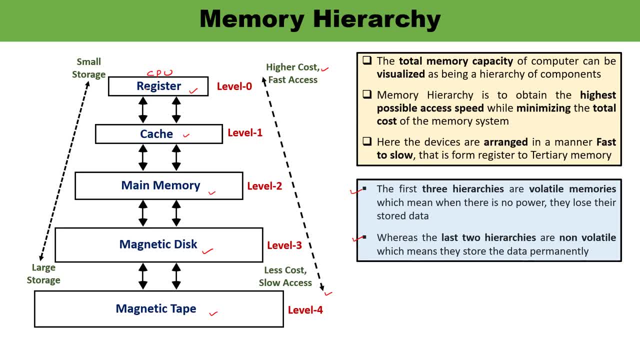 registers are present inside the CPU. since registers are inside the CPU, it means they have least excess time and registers are most expensive and smallest in size, generally in kilobytes, and they are implemented by using flip flops. second level one which is about the cache, so cache memory that is used to store that part of the program which are frequently accessed by. 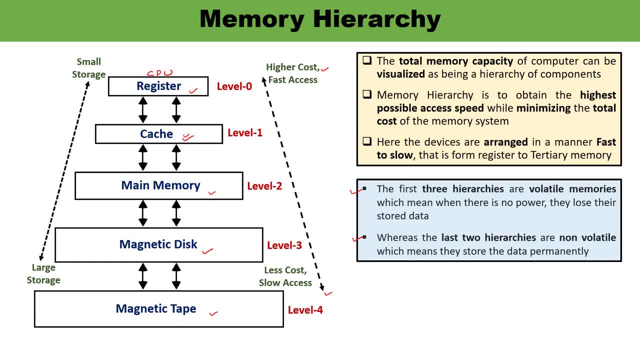 the processor so that frequently accessed program part is being stored in the cache. and this is expensive and smaller in size, generally of the order of the megabytes, and implemented using static ram. level two is about the main memory, or primary memory. it directly communicates with cpu and auxiliary memory devices through io processor you have seen in the previous. 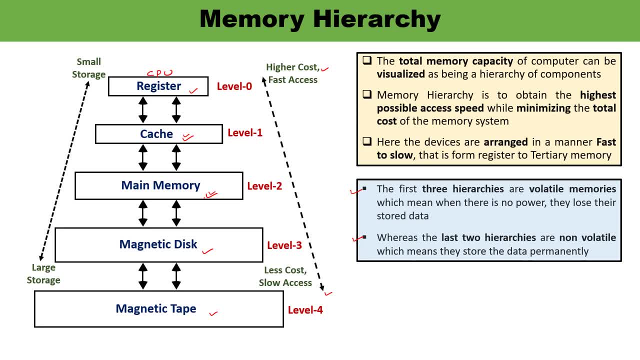 diagram and it is the main storage unit of the computer right and this is implemented using dynamic ram, now level three, that is associated with magnetic disk. it is also known as a secondary storage. so secondary storage devices like magnetic disk, they are present and they are used as a. 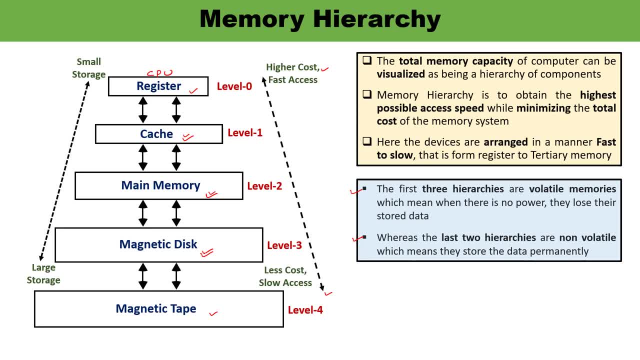 backup storage. right so magnetic disk in the computers. they are usually fabricated by using some circular plates and that has been mounted on a spindle and accordingly it is like implemented, while level four- that is also known as a ternary storage, or this- is associated with the magnetic. 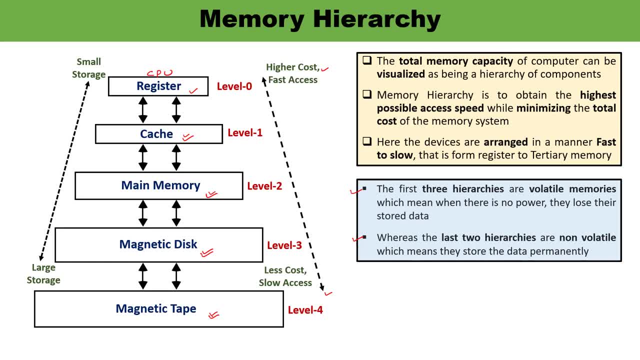 tape, so magnetic disk, is used to store the memory of the computer and that is also known as a backup storage unit. so magnetic tape, they are mainly used for backup data when there is a requirement to store, to take backup of the huge data, and they are used to store removable files.